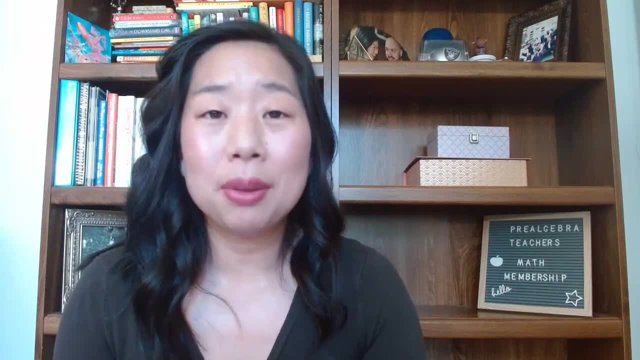 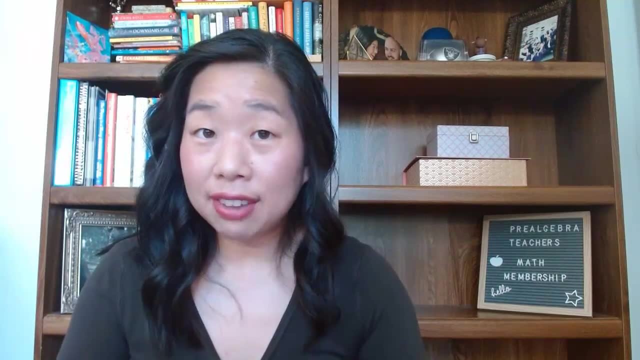 my name is Kathy Martin and I'm the creator of the Pre-Algebra Teachers Middle School Math Membership- your one-stop shop for everything you need to teach 6th, 7th, 8th grade and Algebra 1 math. So shall we dive in? I'm going to be sharing with you my three favorite middle 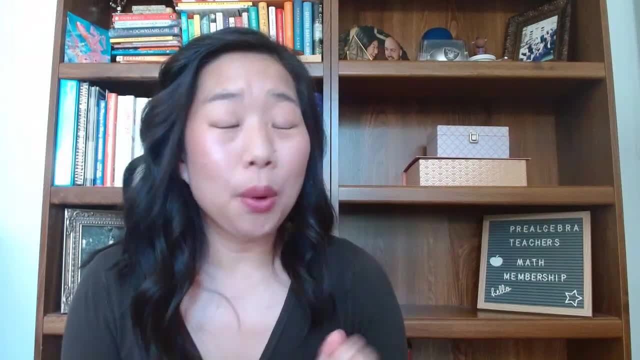 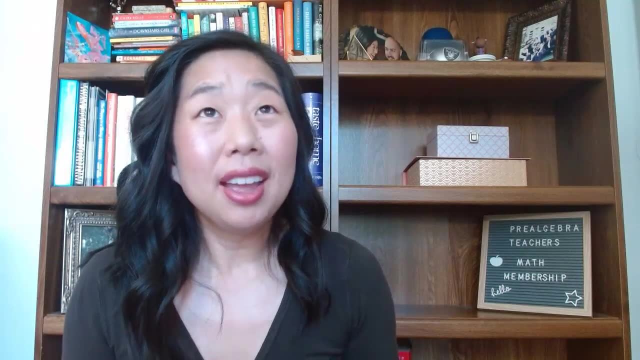 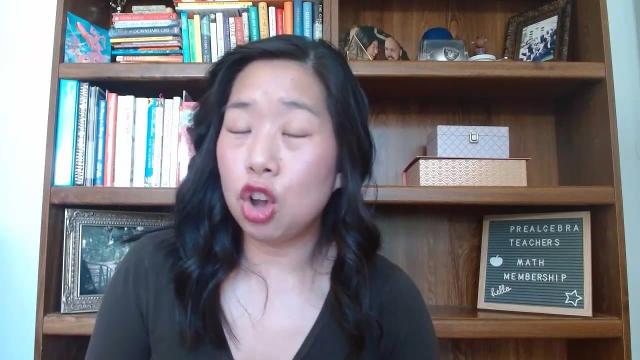 school math activities and games that are totally free. All right, so here we go. Number one, The first one that I think is super underrated, that not a lot of people use- well, I think we just forget about it- is the power of using dice. You can use dice in so many ways, Granted it can be. 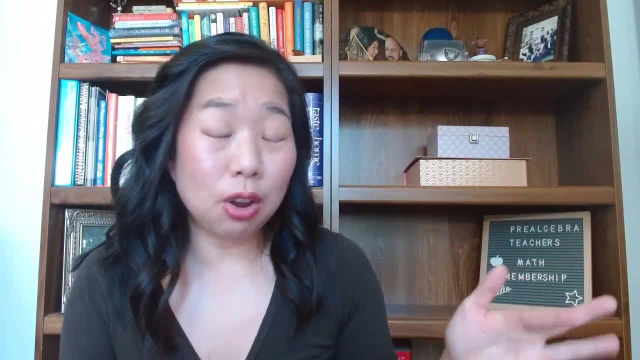 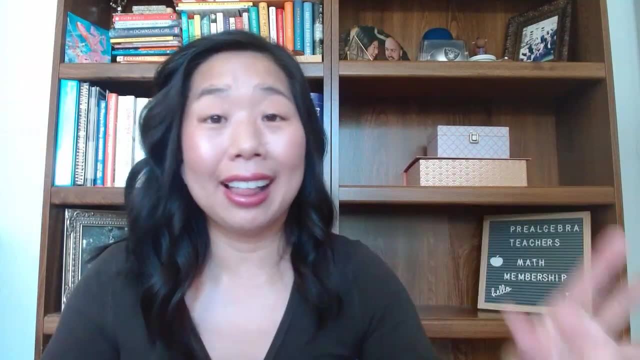 loud. So what I like to do is actually have my students open up their textbook and roll their dice into the textbook. so they don't, so you're not hearing like the clackety-clack-clack-clack of the dice in your classroom all day long. I don't know about. 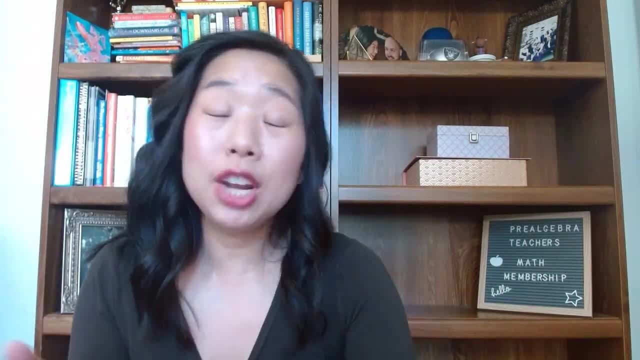 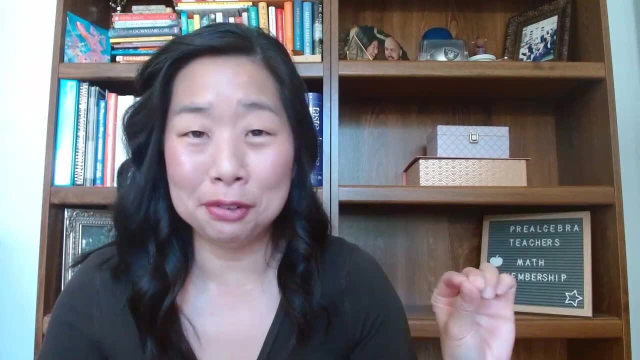 you, but I'm super sensitive to noise And so, anyway, I will have students open up their books so they're rolling it like on a thick textbook just filled with paper, so you don't really hear it at all. It's beautiful And you can use dice in so many ways. You could have, you know, like. 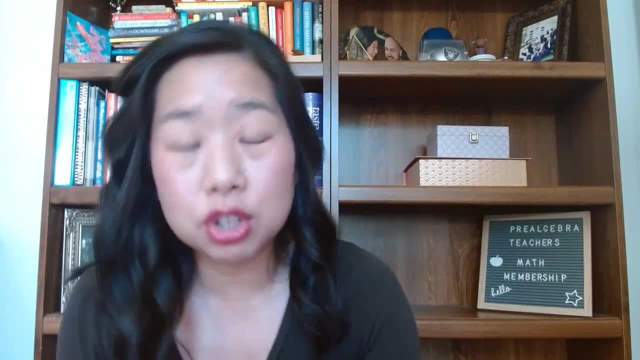 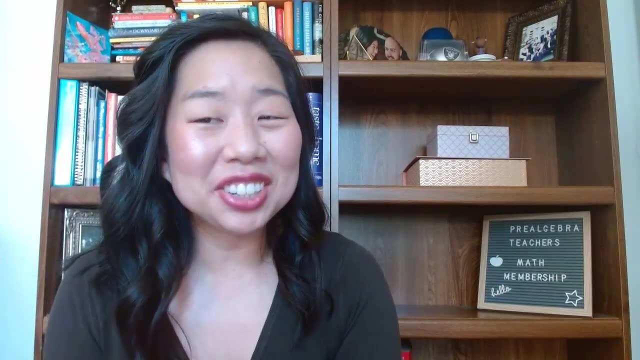 roll two dice and have your students multiply the two numbers that they see, or add the two numbers and then multiply. If you want to get really wild, you can go online and buy multiple like more than six-sided. a six-sided die Like. 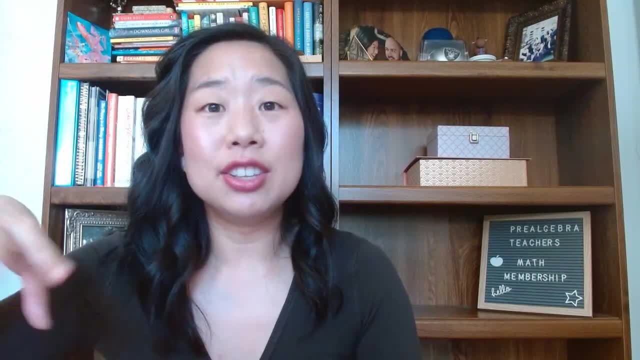 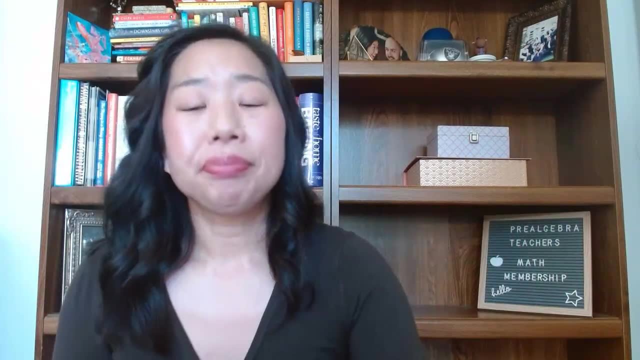 I have seven-sided, eight-sided, ten-sided die And so, like you can, the numbers increase, obviously with the more sides, So you get more than just one through six. But even if you don't have that ability and you have just 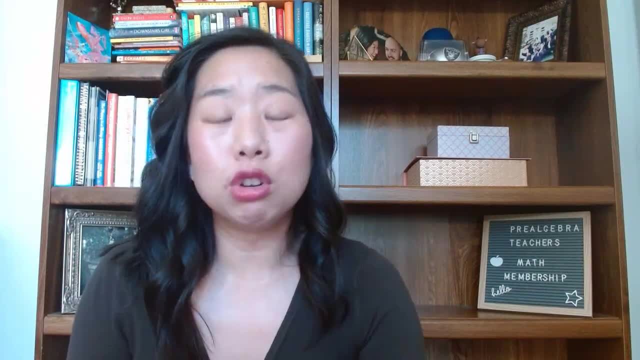 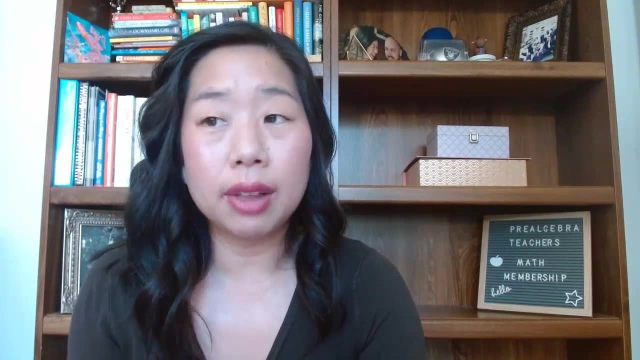 regular dice. you could tell your students, like: okay, we're going to start by multiplying the numbers that you see every time you know two numbers roll or go up, Or you could. and then you can lead to like: okay, we're going to multiply it, but now, every time you see that number, it's. 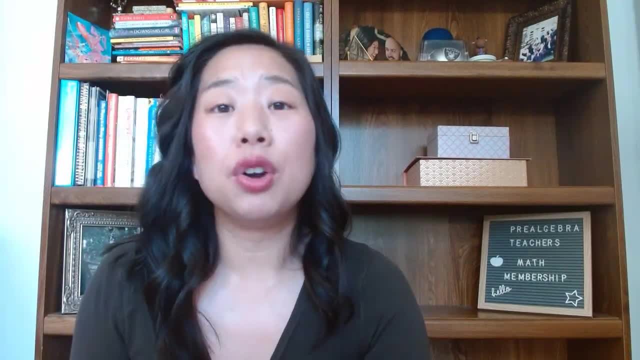 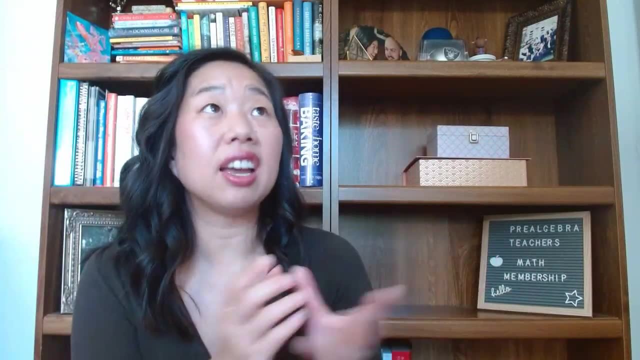 going to double, So that six is going to turn to a twelve. So if you have like two sixes, it's going to be twelve times twelve, Or you could, you know, come up, I like to even put like: 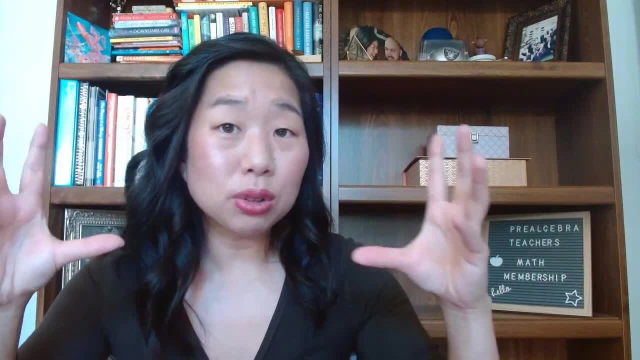 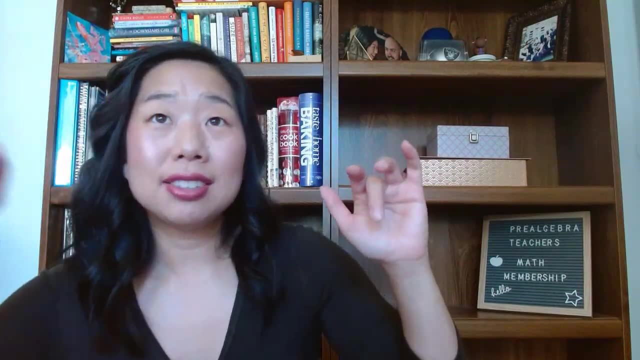 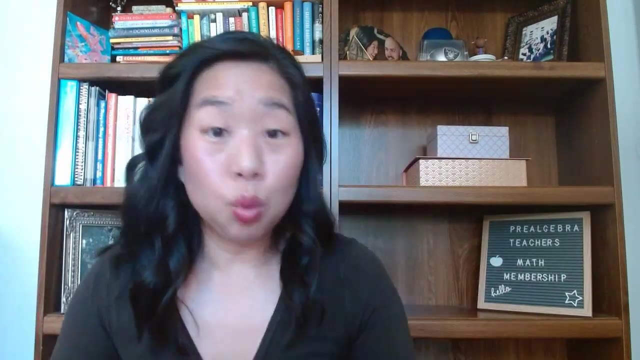 like sentence, mathematical sentence, frames on the board, and then you can like multiply it, Like, so it'll say blank divided by blank plus blank, okay, And then they will roll the die and they will plug in the numbers into that number sentence and then work out, work it out So. 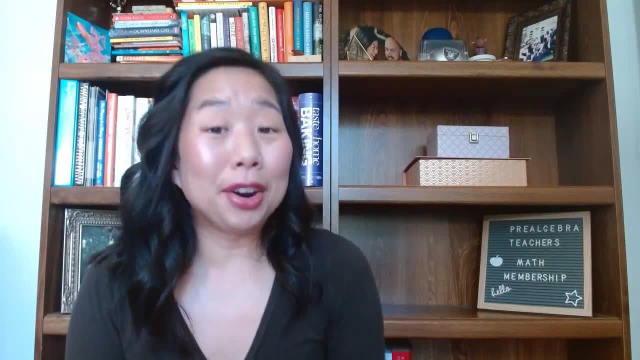 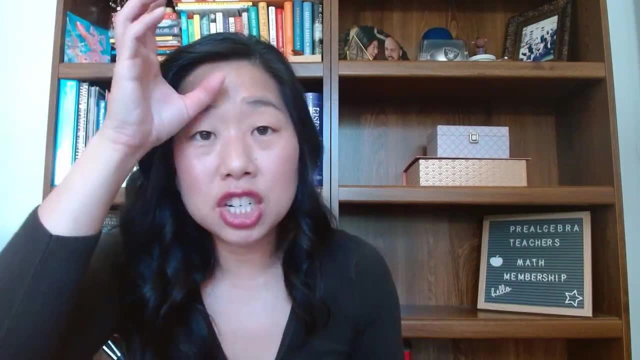 underrated. I'm sure there are a ton of YouTube videos out there that can show you better than me how to use dice for the classroom. but check and check them out. I mean, I don't have any major, I don't have any recommendations, but dice, super underrated and super fun. 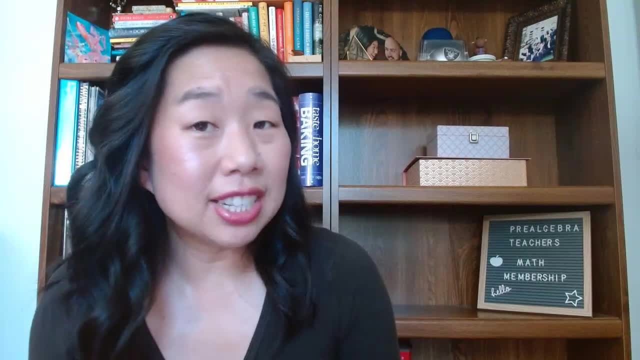 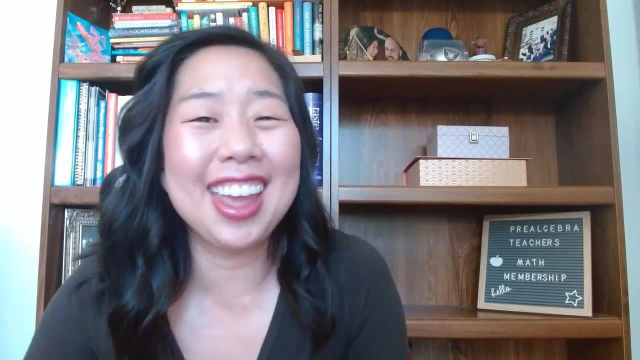 Number two activity: Kahoot and quizzes. I've said this before in some of my other videos, but I love Kahoot- Who doesn't? I mean the Kahoot music itself is fire and the kids love it, but really I love. 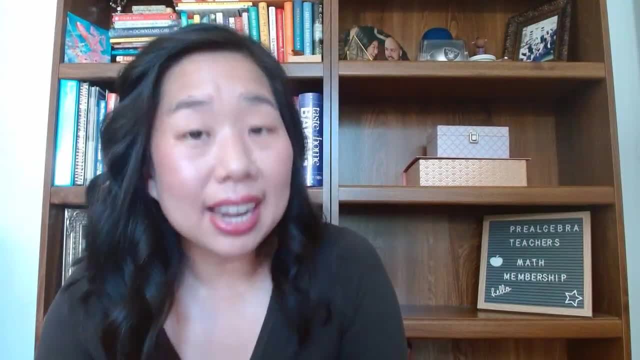 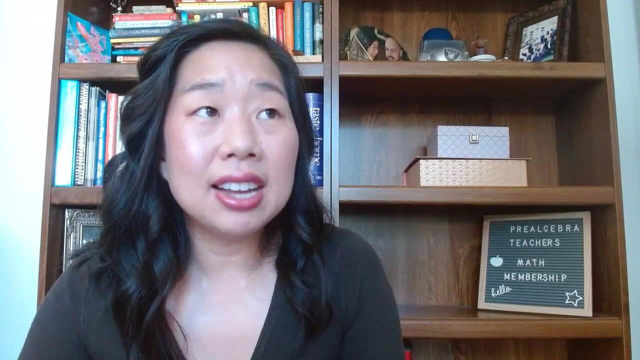 quizzes, And I know that there are a ton of other platforms like this out there. but I am really partial to quizzes because really the big thing that I love about it is it's not. it's individualized, So students don't have to feel like they have to hurry or they have to be in a 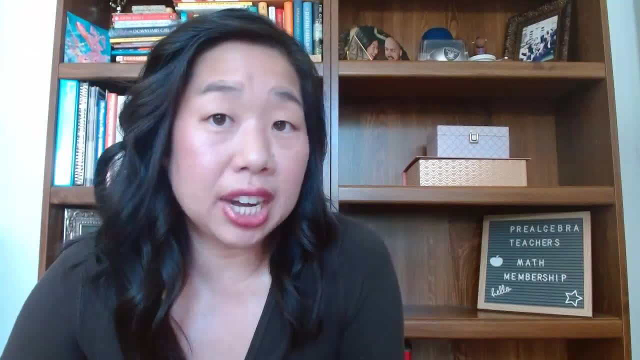 rush. They're not going to be in a rush to do a quiz. They're going to be in a rush to do a quiz, rush to complete whatever question that we're giving them on the screen, because we all know as good math teachers, it is not about speed math. it like speed is. 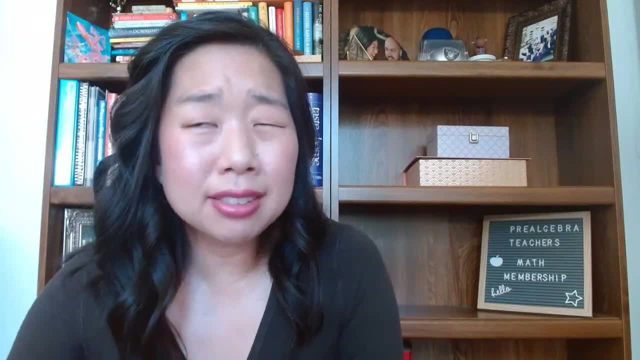 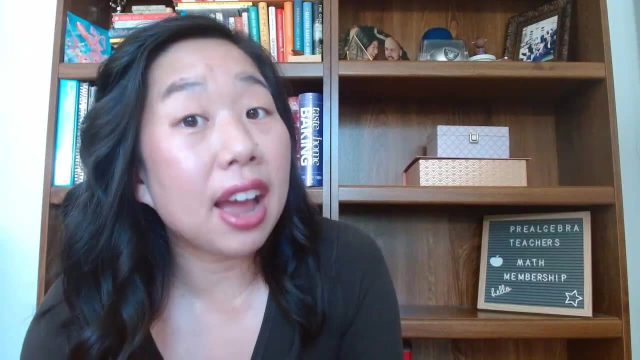 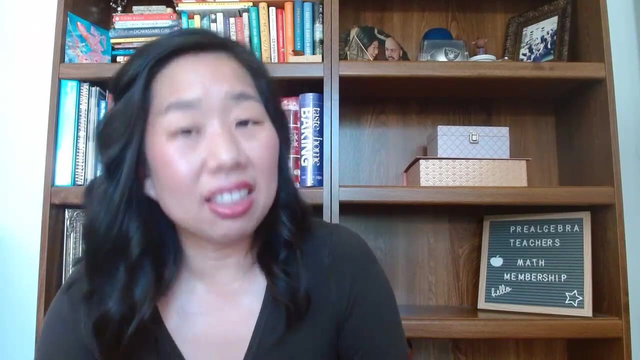 the last thing that we should be encouraging: in math, sometimes speed like we need to be speedy, but for me anyway, I always stress the importance of accuracy and that's why I love quizzes so much is because students who need that extra time can get the extra time. finally, my other favorite activity, that is totally 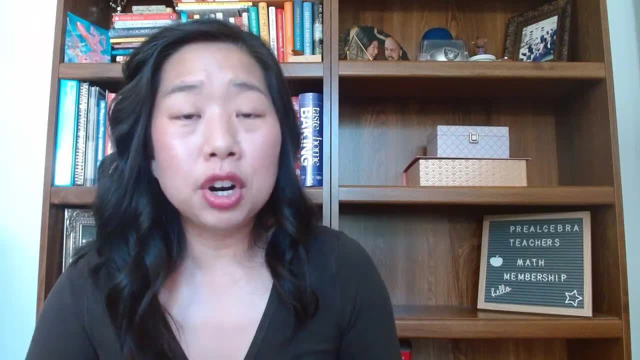 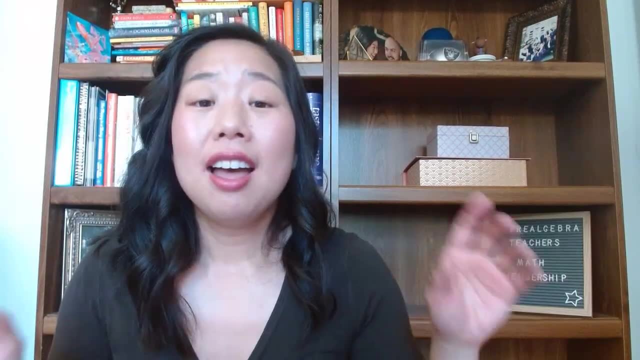 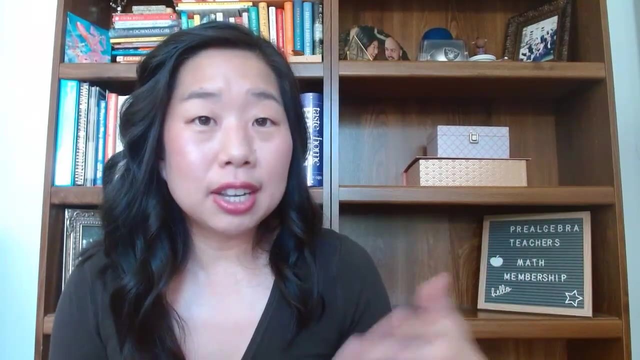 free is a, an online platform or an online game called Wordle for math, and if you've had ever played Wordle before, which is from the New York Times, or I guess the New York Times bought it- I play every day on my phone. still, where you have to like, guess the five-letter word of the day, this is Wordle for math. 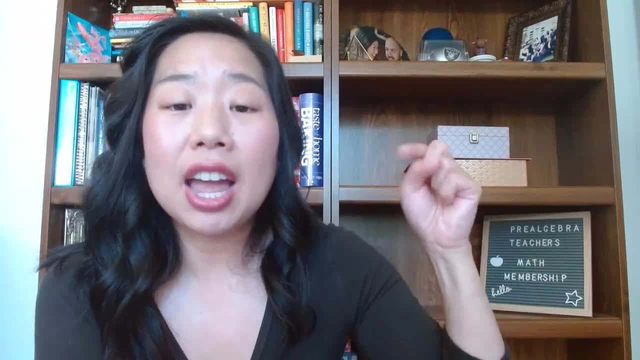 and it's a great way to get the extra time. and you can get the extra time if you want to see this in action. I actually have a YouTube video for it that I will include the link in the description box to actually show you how it works, what.